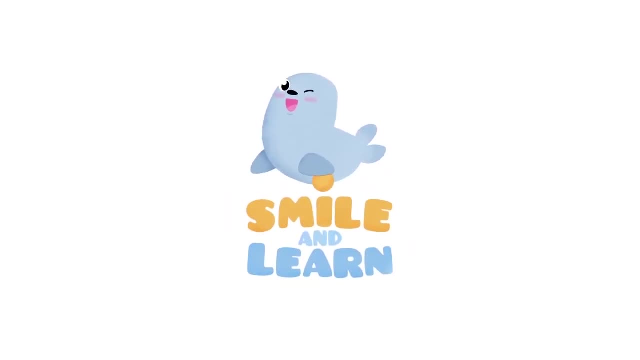 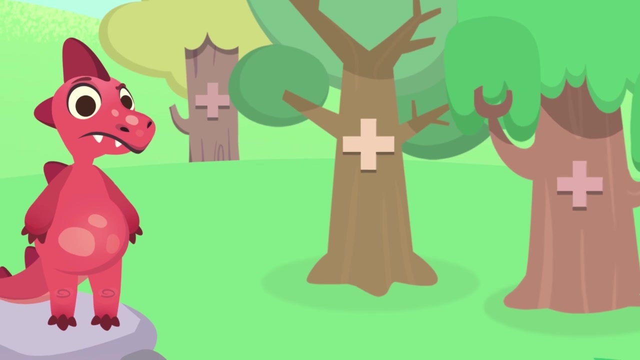 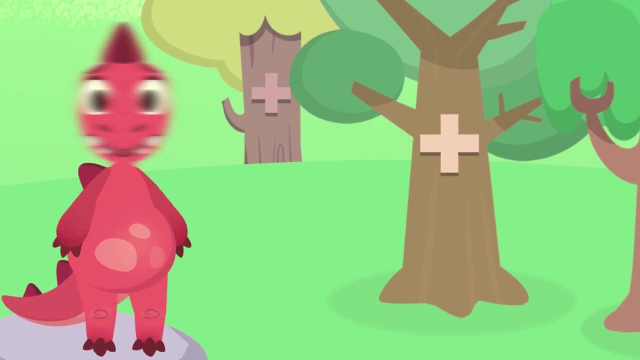 Hey, Dino, What's the matter? I see you're worried. Do you know what all these crosses are for? You don't? That's the plus sign for additions. Do you know how to add? Don't worry, Dino, I'll teach you how. 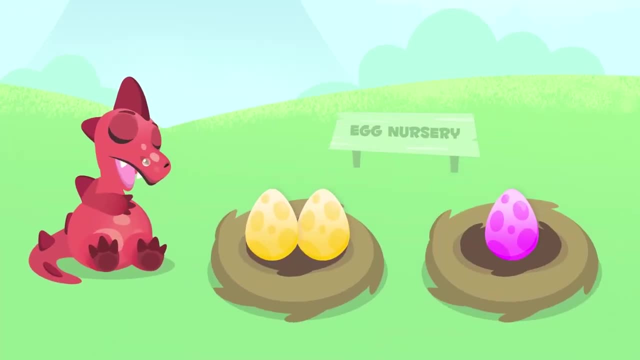 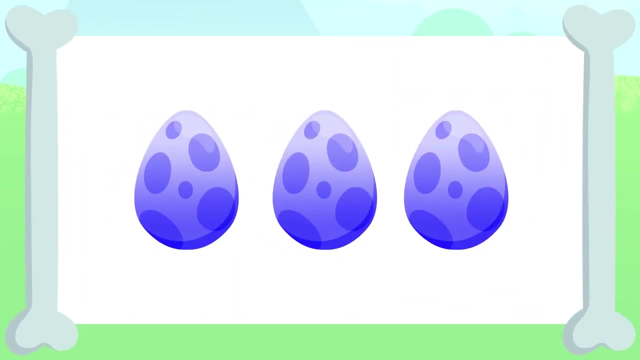 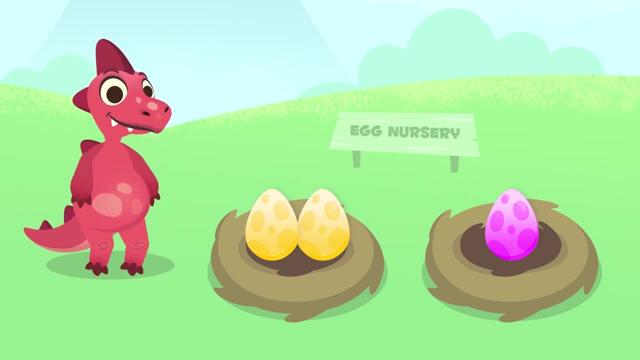 Hey, Dino, wake up. You have to look after all these eggs. Do you know how many are there? Let's add them up. Adding up means putting together or grouping together several things. Today we're going to add up Dino's eggs. Are you up for it? Let's see how many eggs there are. 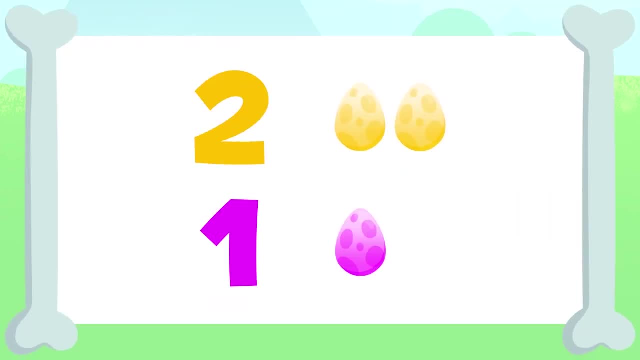 Up here we have one and two and down there we have one. So all together they sum one, two and three, Three. There are three eggs. Two plus one equals three. We have completed our first addition. Adding up two plus one gives: 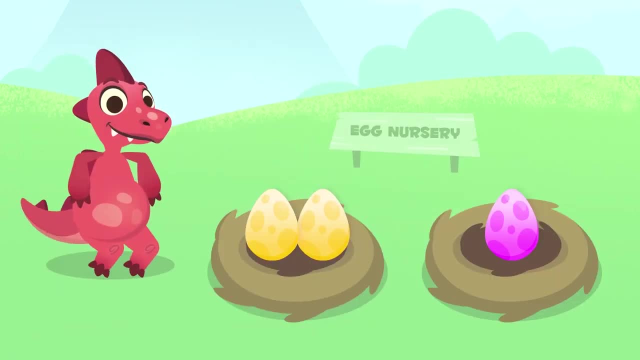 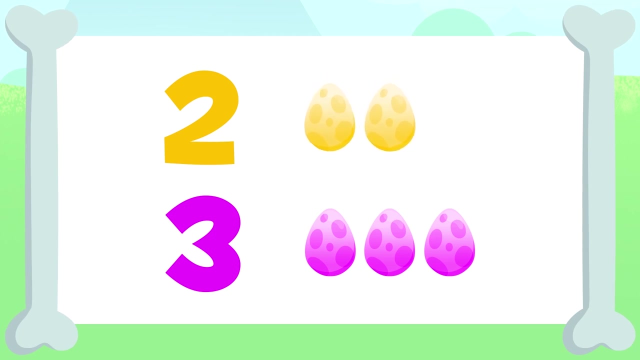 you three. This has been your first addition. Dino, Are you happy? Wow, it looks like you have more eggs to look after. Do you know how many eggs are there now? Shall we add them up? Up here there are one and two eggs, and down there we have one, two and three eggs. We have to add two plus. 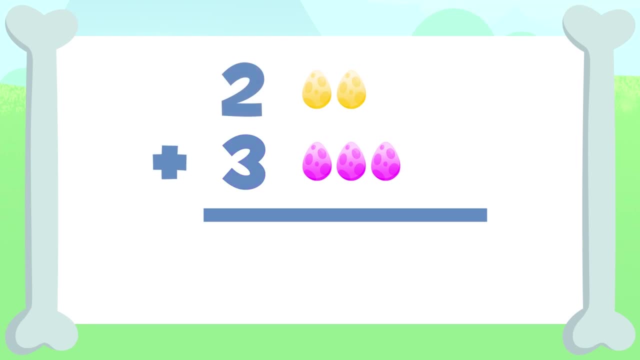 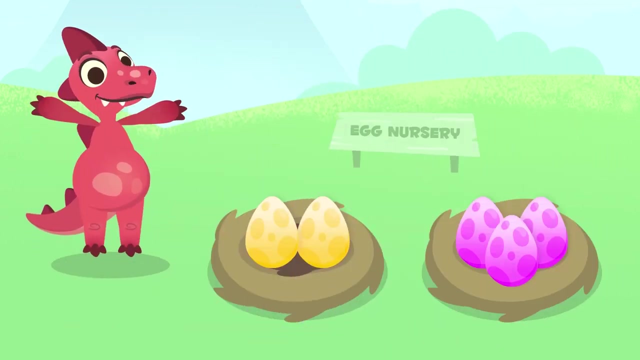 three. So all the eggs together would sum up one, two, three, four and five. We have five eggs. Two plus three equals five. The result of adding up two plus three is five. Well done, Dino. Do you like adding up? Whoa more eggs are falling down. Let's add them up to find. 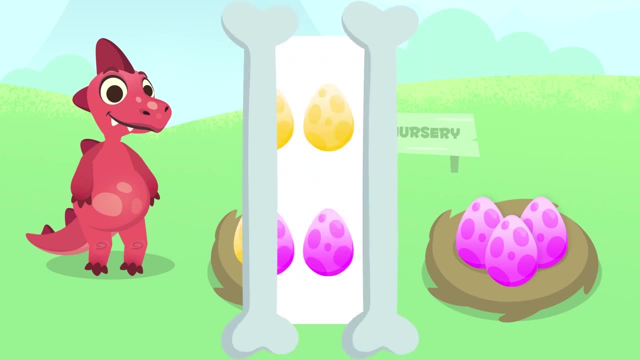 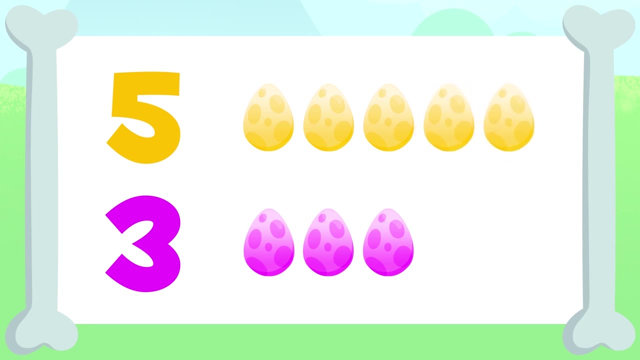 out how many eggs in total you'll have to look after. okay, Up here there are one, two, three, four and five eggs, And down there we have one, two and three eggs. We have to add five plus three, So the result is one- two. 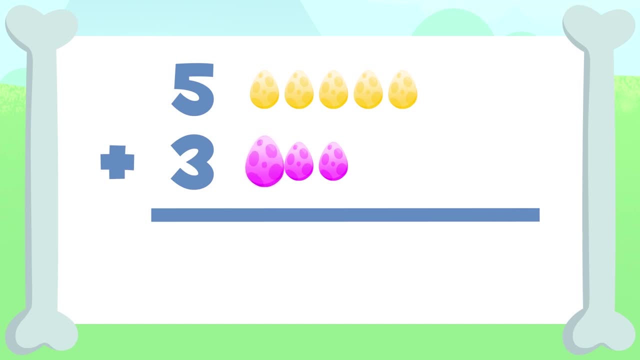 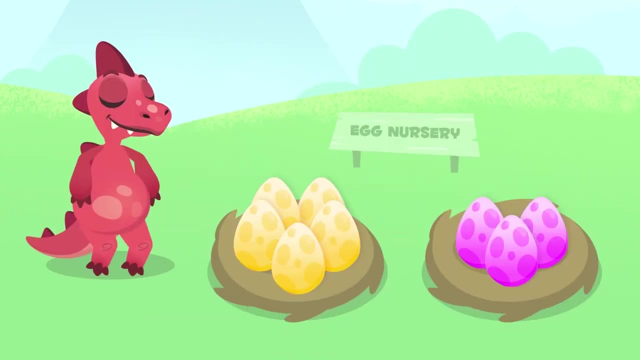 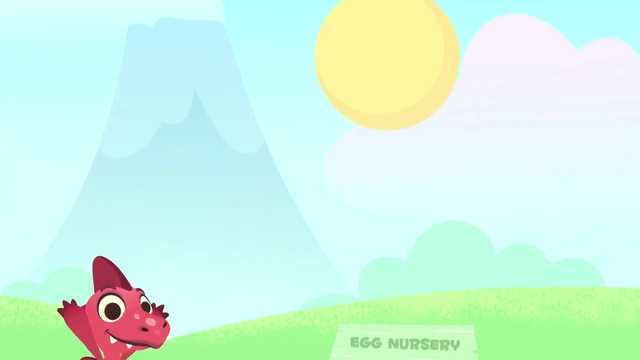 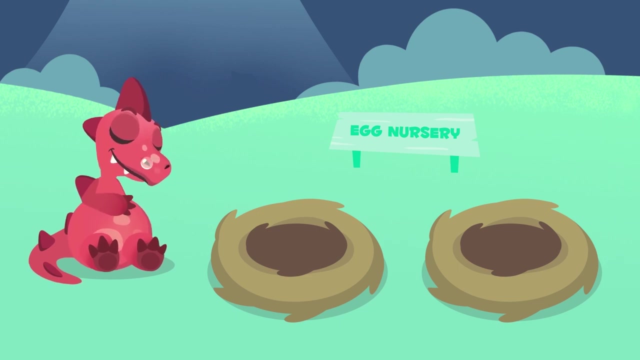 three, four, five, six, seven and eight. We have eight eggs. Five plus three equals eight. Well done, Dino. Today you need to look after eight dinosaur eggs. Now you know how to add up. You've fallen asleep again, Dino. wake up. everyone's gone. You're not much of a dinosaur. 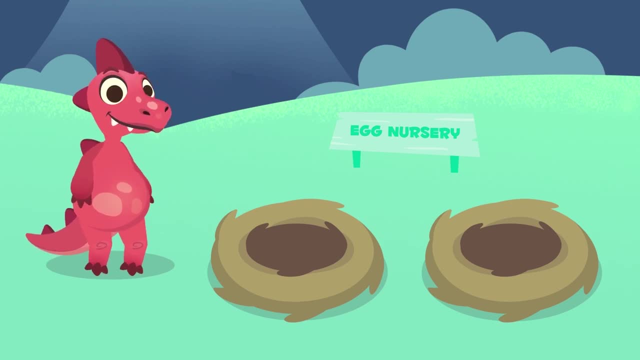 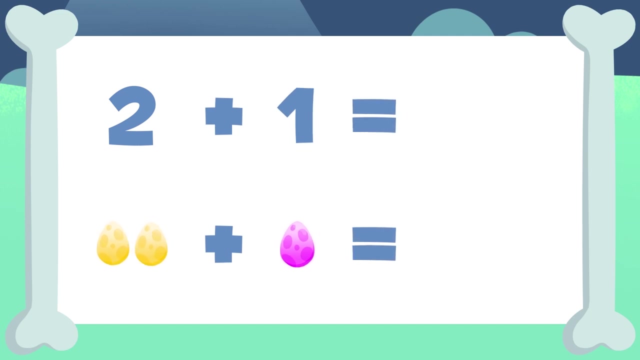 or Egg Guardian, are you? Well, it's okay, Dino. Today we've learned how to add. Do you want to recap? We could also do horizontal additions. It's done in the same way. Pay attention: 2 plus 1 equals 1,, 2, and 3.. 2 plus 1 equals 3.. Very well, Let's do the next one. 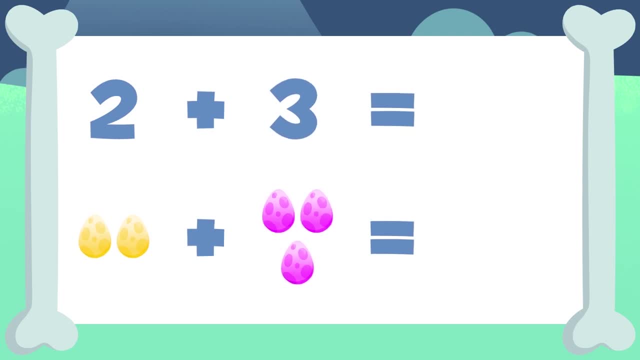 2 plus 3 equals 1,, 2,, 3,, 4, and 5.. 2 plus 3 equals 5.. Way to go, Let's do another one. 5 plus 3 equals 1,, 2,, 3,, 4,, 5,, 6,, 7, and 8.. 5 plus 3 equals 8.. So good. 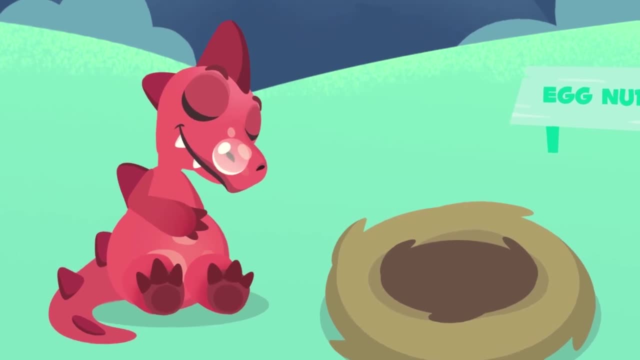 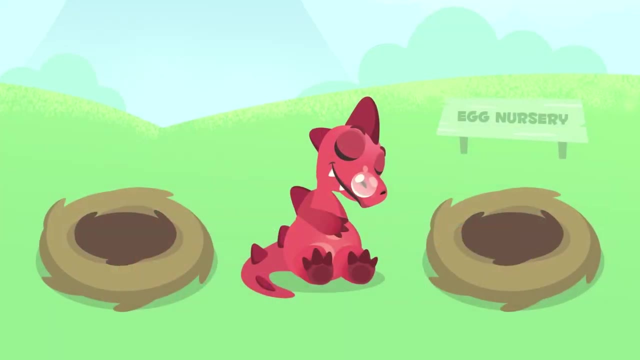 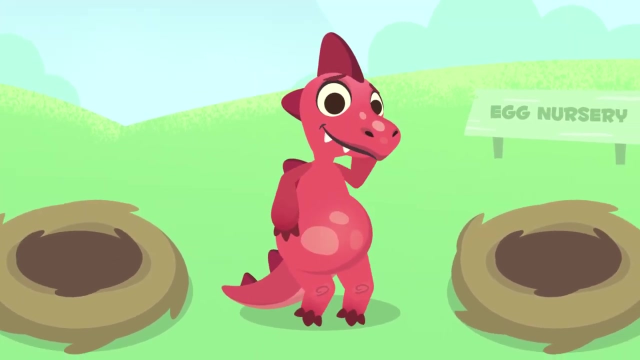 I'm afraid. I'm afraid there's nothing we can do about Dino. He's had a hard day, so we'll just let him sleep a bit more. See you around everyone. Hey, Dino, You fell asleep again. My my, I see you're not doing much. 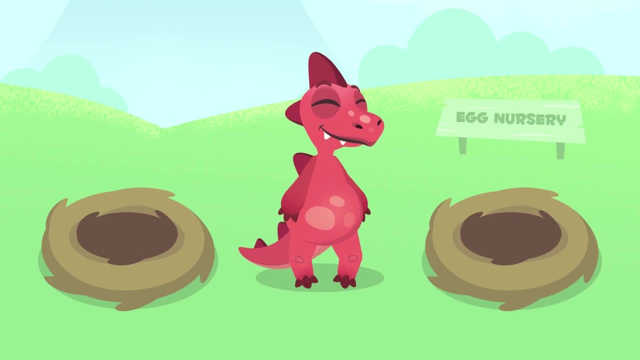 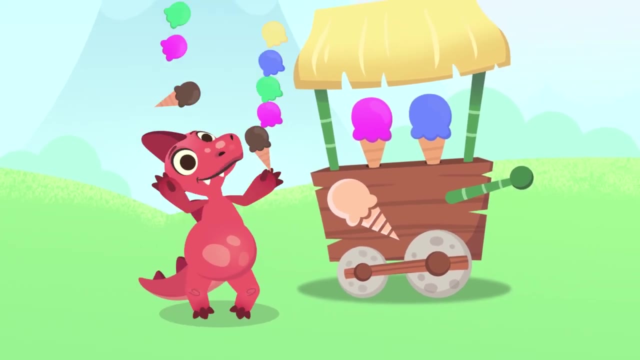 Are you bored? Let's go get some ice cream. Whoa Dino, You got yourself two huge ice creams. It'll take you long to eat, and both. Wow, you were really hungry, weren't you? Now that we're full, 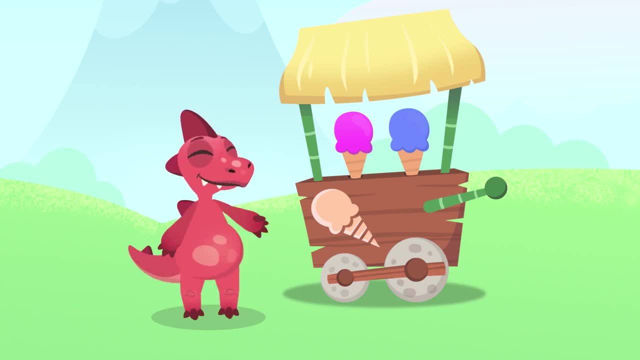 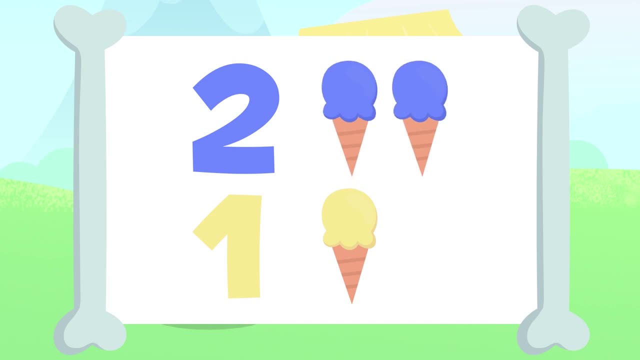 we can practice additions. What do you say? Come on, let's add. How many ice creams are there? Up here we have one and two and down there we have one. Go ahead, You do the adding. I'll give you a few seconds. 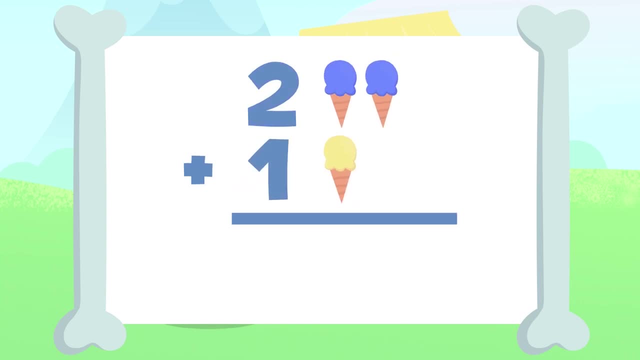 You got it. Let me try. All ice creams together would be one, two and three Three. There are three ice creams. Two plus one equals three. We just did our first addition. The result of adding two plus one is equal to three. 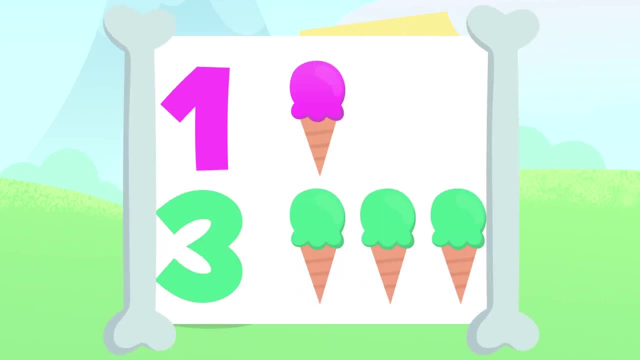 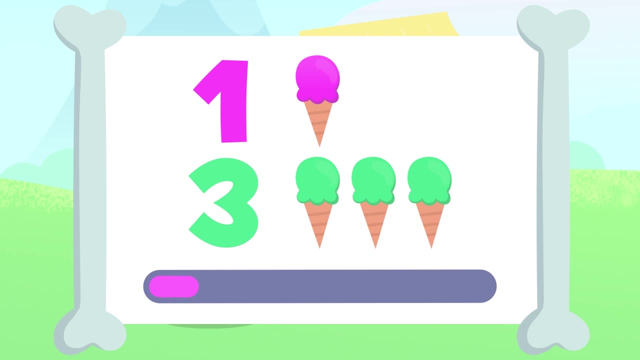 Well done, Dino. Let's try another one. There's one ice cream up here and three down there. Why don't you add them up? Take your time, You got it. If we add these ice creams together, we'll have in total one, two, three and four- Four. We have four ice creams in total. 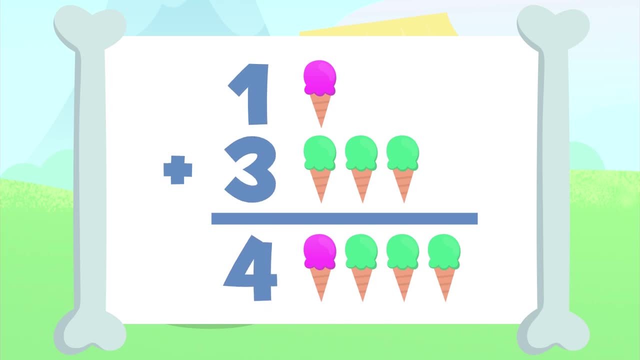 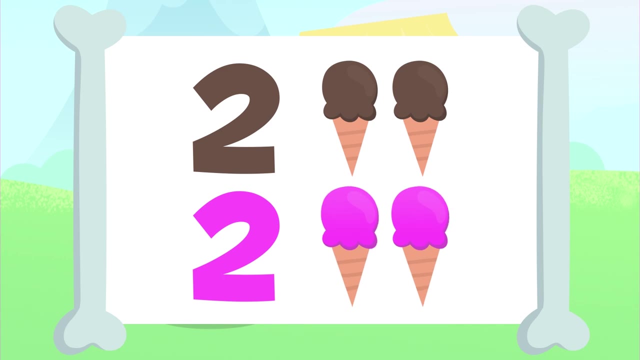 One plus three equals four. Shall, we carry on. Now you'll have to add these two ice creams together. We'll add these two ice creams up here to those two ice creams down there. I'll give you a few seconds to add them up. 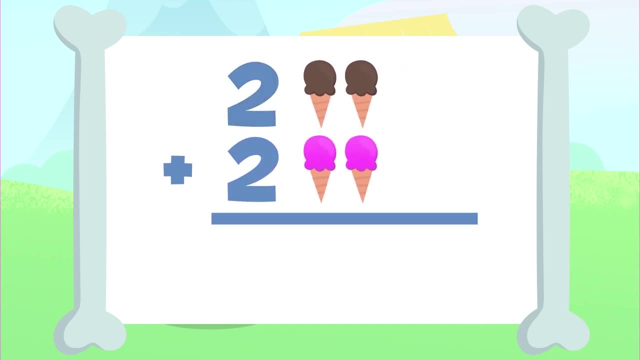 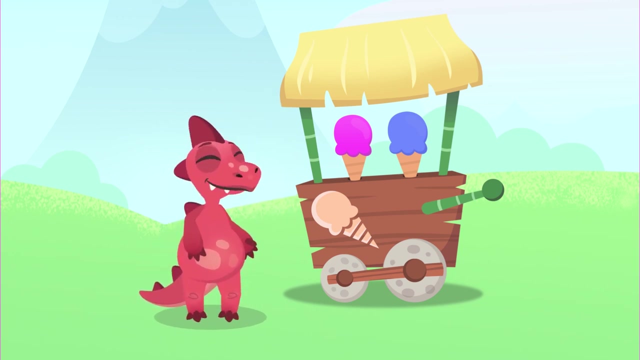 How did that go? You got it. The result of adding up two plus two is one, two, three and four, Four. There are four ice creams. Two plus two equals four. Let's try another one. You'll have to add these four ice creams up here to the one ice cream down there. Let's go for it. 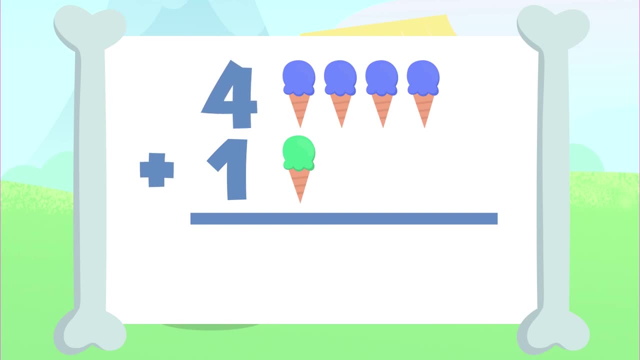 You got it. The result of adding up four plus one is one, two, three, four and five- Five. We'll add these three ice creams together. That's cool, You got it. The result of adding up four plus two is one, two, three and five, six. 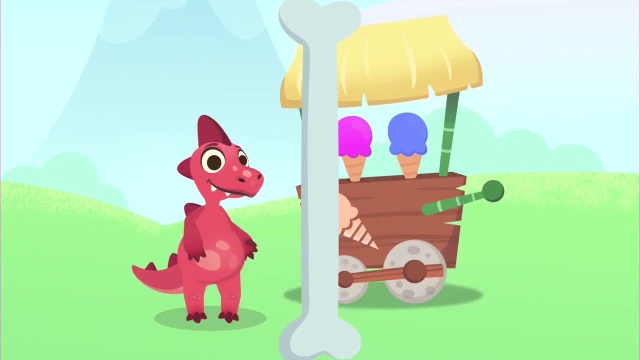 You got it. The result of adding up the three plus two is one. Great, Now you'll see what it looks like. Can you guess where the last ice cream came from The last place? We have to get them up here so we can put those two down. 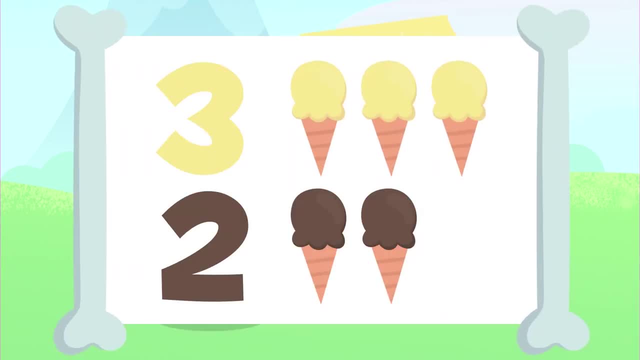 The last place. Now we need to add the next ice cream together. Do we need to add theúde? No, our last color is snow. Shall we put on the child? No, You need to add the other one too. We put the last one in. 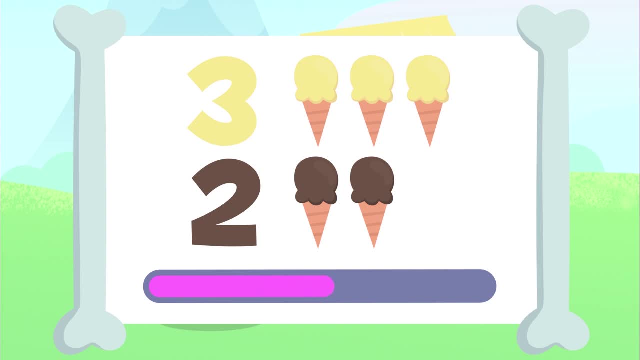 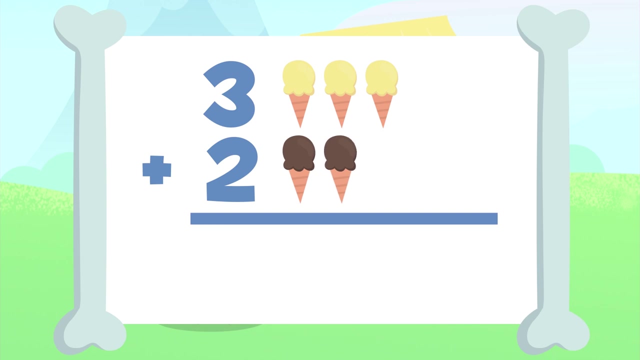 Now we need to do the others. How much ice cream we will have out of this? On all the ice creams, O sets? That's it. The result of adding up 3 plus 2 is 1,, 2,, 3,, 4, and 5.. 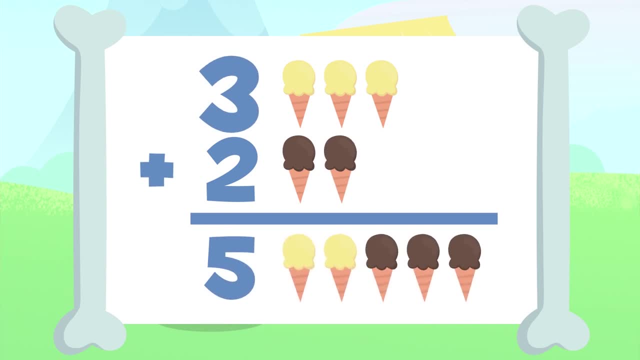 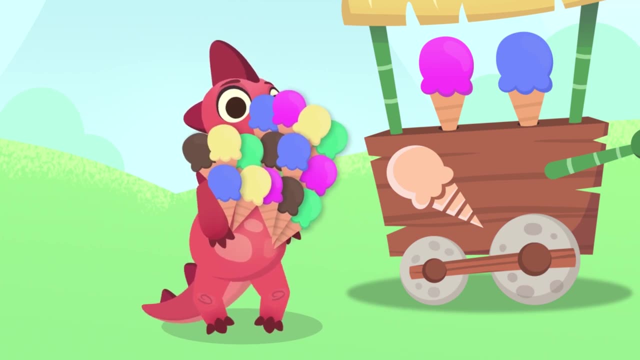 Five. There are five ice creams. Three plus two equals five. And what are you going to do with all this ice cream, Dino? Are you going to eat it? You're going to feel sick, Dino. Wouldn't it be best if you save it for later? 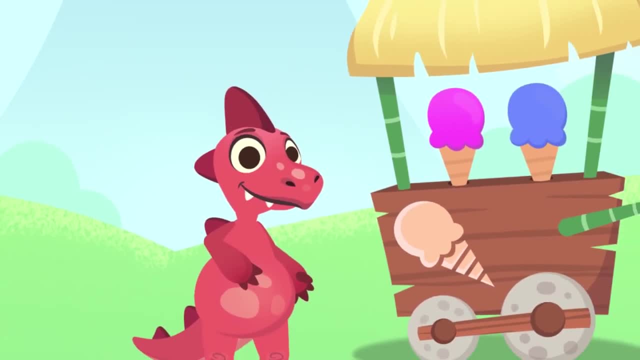 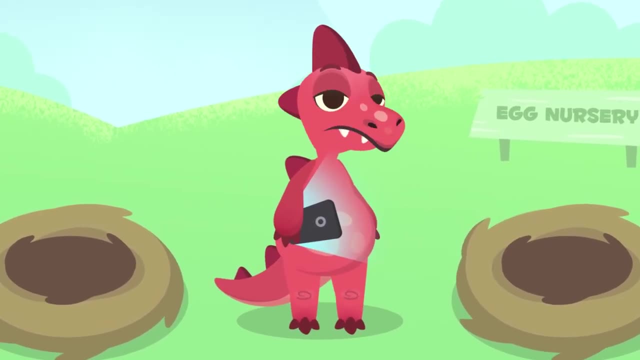 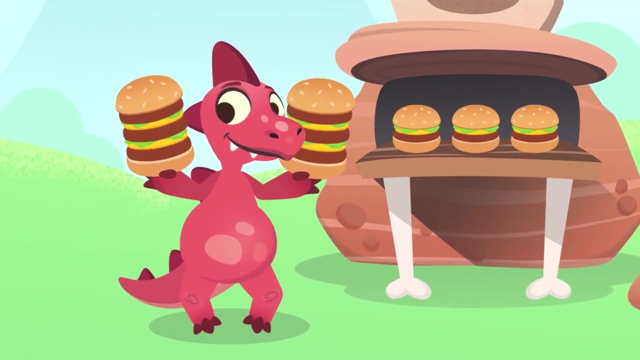 My, my Dino. You're never full. Hey, Dino, How's it going? I see you're not doing much today either. Are you bored? Shall we go get some delicious dinner. Look at those super hamburgers you got yourself, Dino. 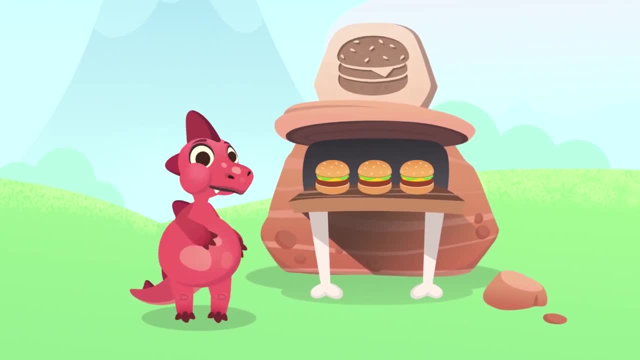 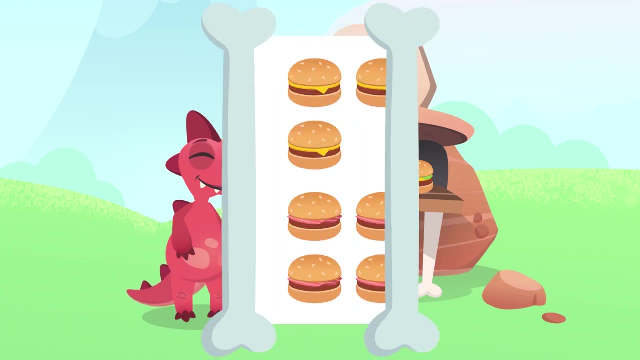 It'll take you a while to eat them. Wow, you really were hungry. Now that we're full, we can practice some additions. What do you think? Come on, let's add. How many hamburgers are there? Up here we have three and down there six. 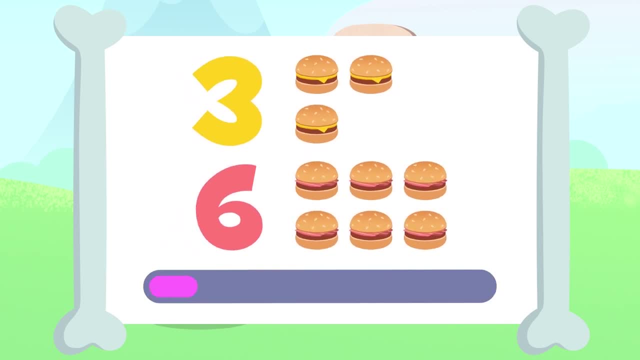 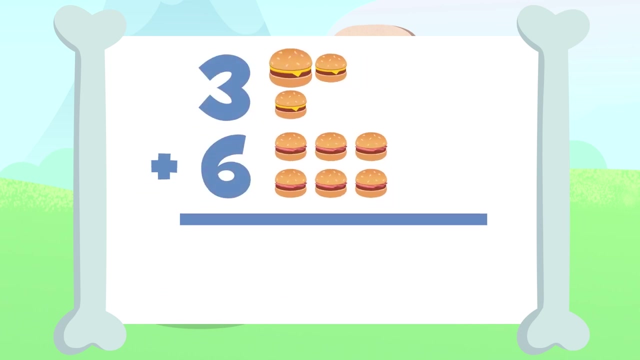 Go ahead, You do the adding. I'll give you a few seconds. You got it. Let me try. All hamburgers together would be one, two, three, four, five, six, seven, eight, nine, nine. We have nine hamburgers. 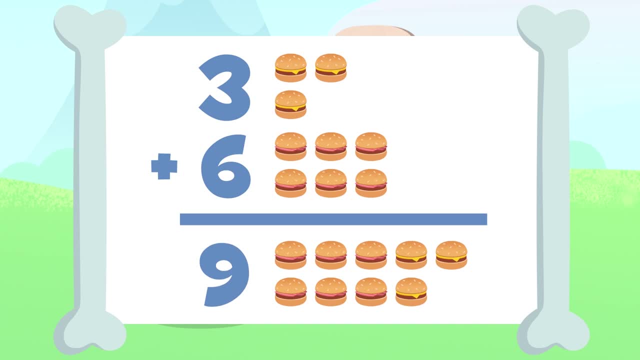 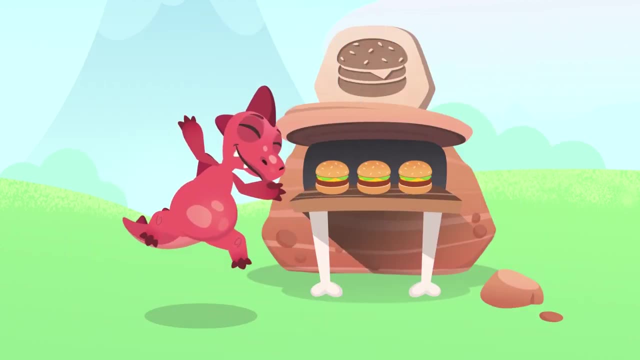 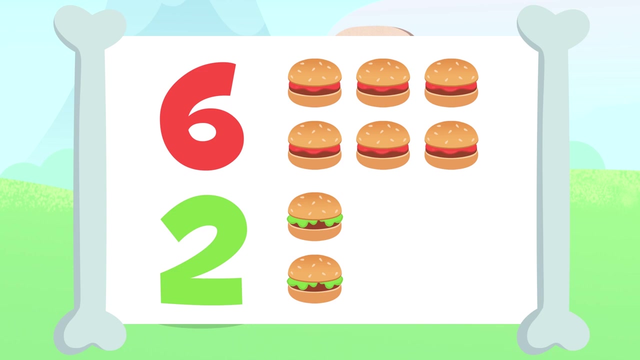 Three plus six equals nine. We just did our first addition. The result of adding three plus six is equal to nine. Well done, Dino. Let's try another one. There are six hamburgers up here and two down there. Why don't you add them up? 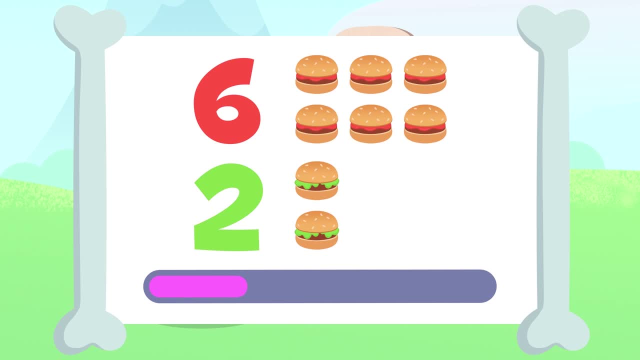 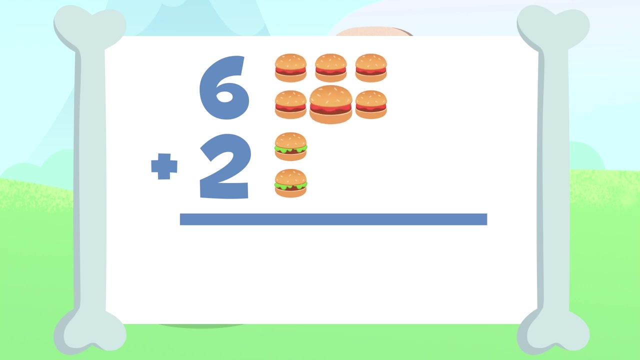 Take your time. Are you ready, Dino? Yeah, You got it. If we add up these hamburgers, we'll have one, two, three, four, five, six, seven and eight Eight. We have eight hamburgers in total. 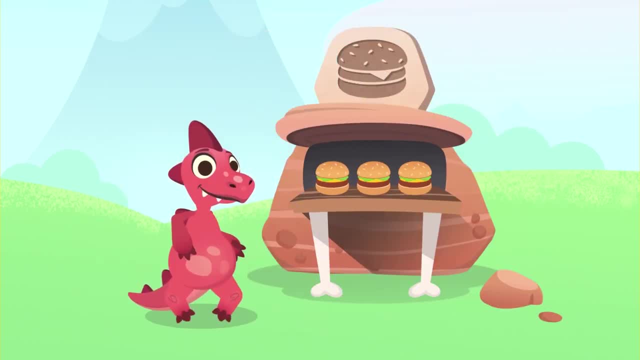 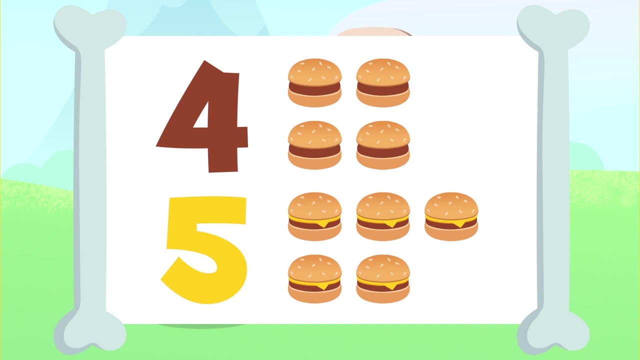 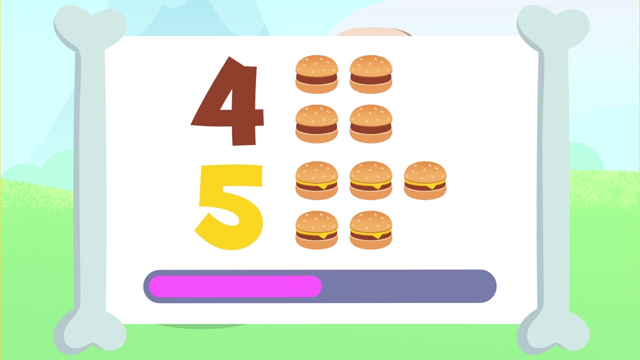 Six plus two equals eight. Shall, we carry on. Now you'll have to add these four hamburgers up here to those five hamburgers down there. I'll give you a few seconds to add them up. How did it go? You have it.